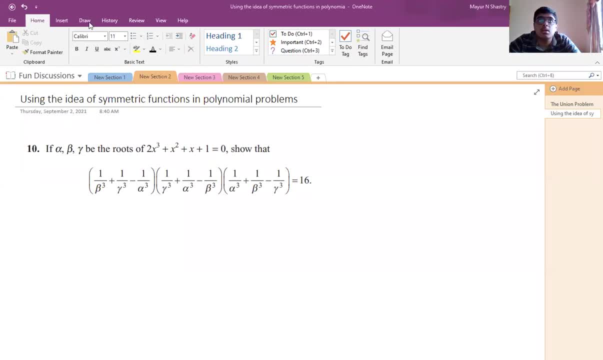 Hello everyone, I welcome you to another mathematical fun discussion. So today's video is going to be about symmetric functions and how do we use them in polynomial problems. So first let us learn what exactly are symmetric functions. So let me explain through some examples. say something like this: 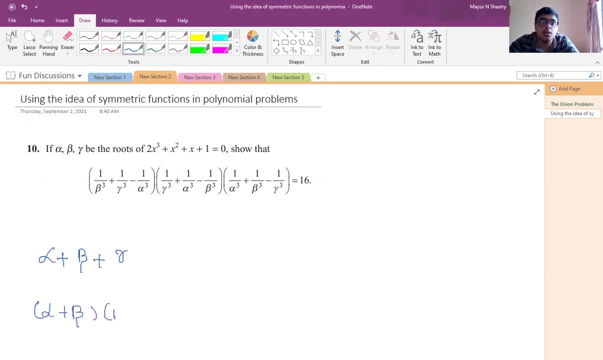 maybe something like this. So in these expressions, notice that if you change any two of these- alpha, beta and gamma- then the expression remains unchanged. Say, you change alpha and beta, then what is going to happen? you'll get beta plus alpha plus gamma, and it's the same thing. 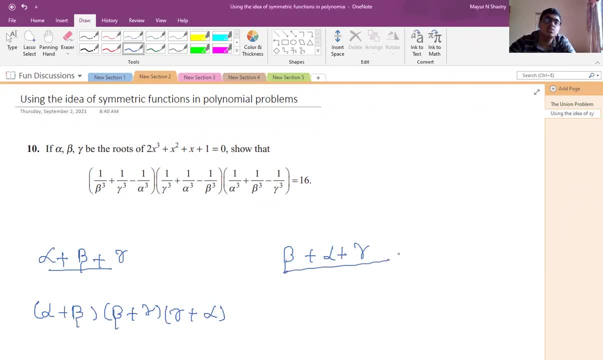 as the cumulative property of addition holds, And here also say you want to replace two of them. say you want to replace alpha and gamma, so you would get gamma plus beta times beta plus alpha times gamma plus alpha. It is the same thing. if you notice you would have to. 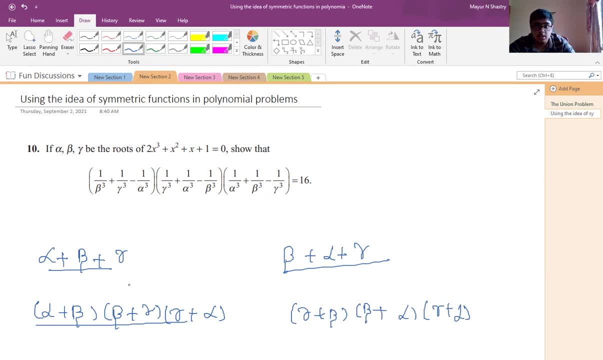 apply the, you know, commutative property of addition and also the associativity of multiplication, So that would give you that these two are the same expressions. So thing is, symmetric functions are those functions where you change any two of the n variables. let us say there are n variables. 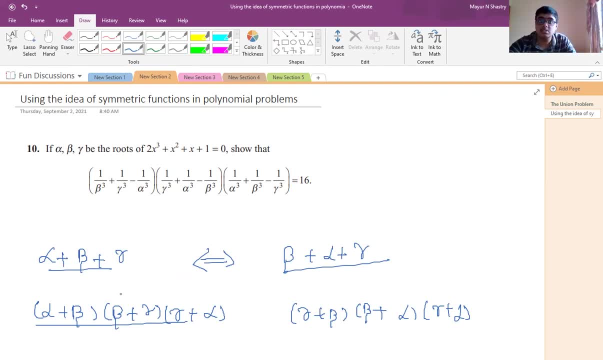 you change any two of them, the expression would remain unchanged. So that is what is: symmetric functions. So we would tackle this problem using symmetric functions. So let us just see what the problem is telling. It's saying that alpha, beta and gamma are the 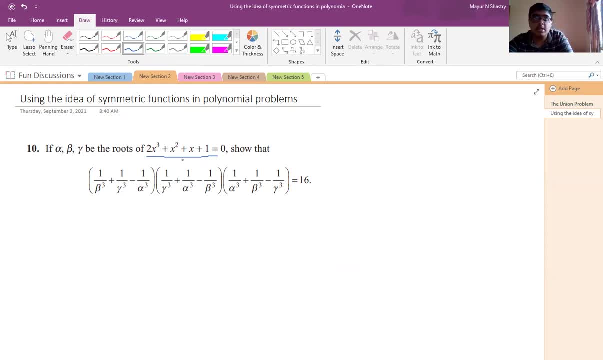 roots of this equation: two x cube plus x square plus x plus one equals zero, and we need to show that this expression- one by beta cube plus one by gamma cube minus one by alpha cube, times one by gamma cube plus one by alpha cube minus one by beta cube, times one by alpha cube plus one by beta cube. 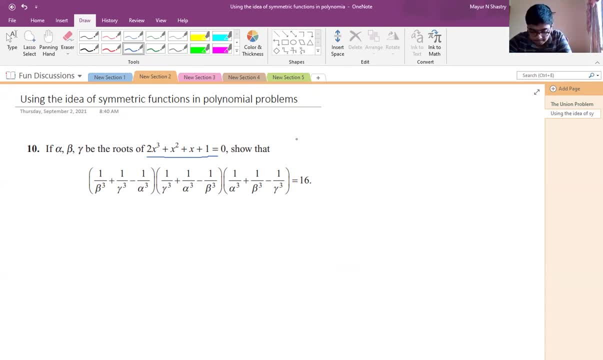 minus one by gamma cube that equals 16.. So you notice that it's a very complicated expression because we have plus and then a minus, and then product. Imagine how many terms you would get if you do it by brute force. that is just multiplying all the terms together. So 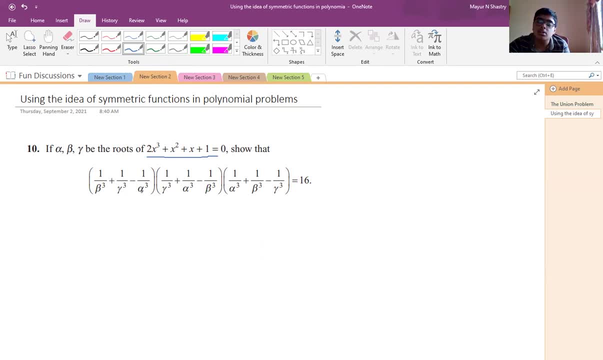 uh, how do you think we can start this problem? You can try to pause this video and think about it and you may get the solution. and yeah, if you don't get, you can watch this video. So realize that this expression is complicated, so I can write this as one by alpha cube plus one by 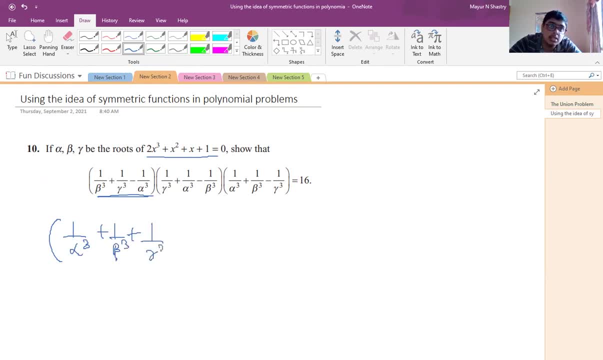 beta cube plus one by gamma cube, minus one by alpha cube, plus one by beta cube, plus one by gamma cube, minus two by alpha cube. why am I doing this? because it's easy to calculate this expression where there are all pluses. that's the motivation. so yeah, this is the same thing again. we're going. 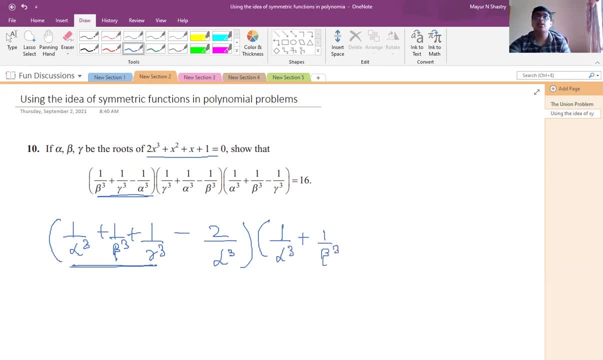 to do one by alpha cube plus one by beta cube. we are adding a beta cube, one by beta cube, because it's a minus here, plus one by gamma cube, minus two b two by beta cube. then again you would have similar one by alpha cube plus one by beta cube, plus one by gamma cube. that minus two by gamma cube. 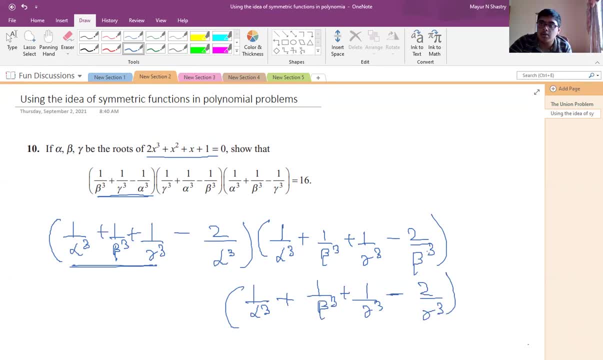 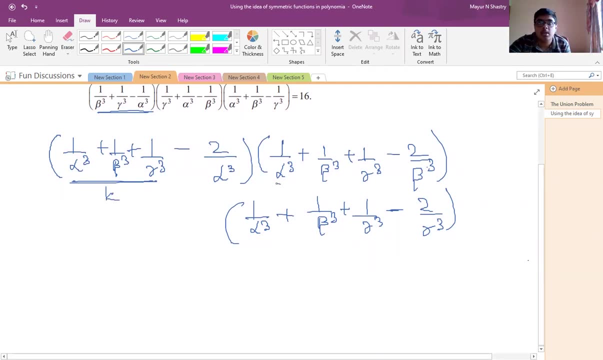 so this is what we need to calculate and what we're going to do is we're going to assume that this is some quantity. let us say k, this is k, this is k and this is k, and we want to find k right. so we need to find this expression, k minus two, by alpha cube times k minus two. 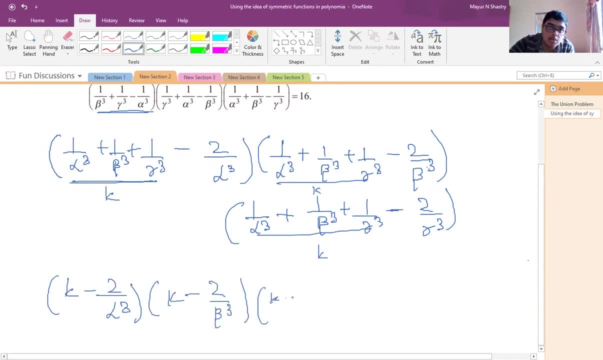 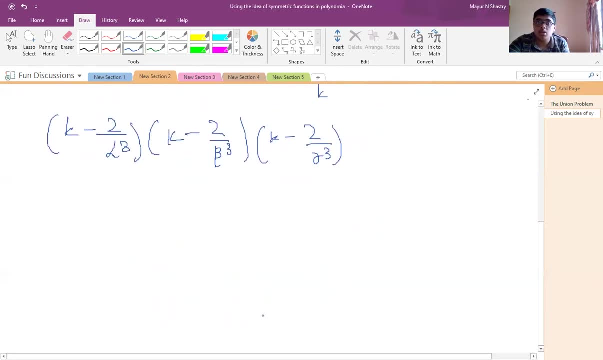 by beta cube times k minus two by gamma cube, and this is not very hard to expand. it's simplified very much. so now our goal is to find out the value of k, that is, one by alpha cube plus one by beta cube, plus one by gamma cube. how do we do that? that's where we need symmetric functions. so 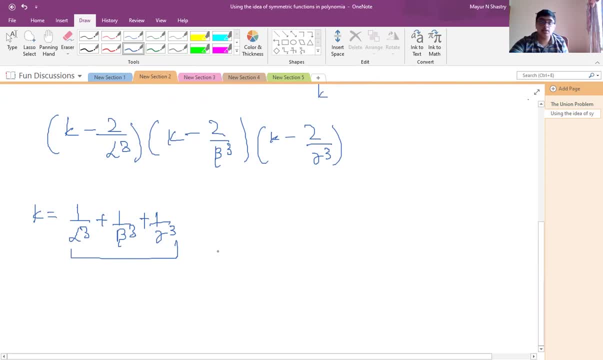 this is, of course, a symmetric function. you change any two of alpha and beta, you get the same expression. it's obvious. so the thing is, we need to find- we need to first find the polynomial with roots, one by alpha, one by beta and one by gamma. first we need to find that, because then only we can use the idea of symmetric functions. 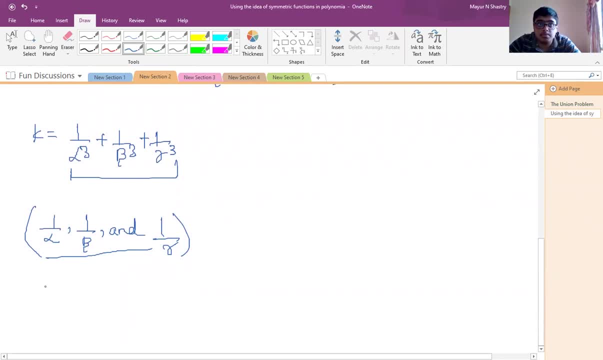 so let us find this. so now, uh, let us, let us calculate the sum of the roots. sum of the roots is just one by alpha plus one by beta plus one by gamma. that equals alpha beta plus beta gamma plus gamma. alpha by alpha beta gamma. so what, what? what is that? okay, so let's go back and see alpha beta plus. 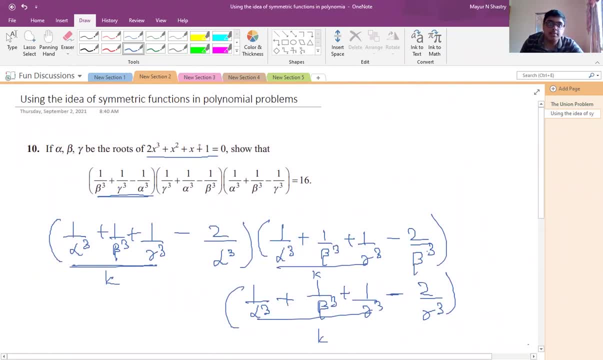 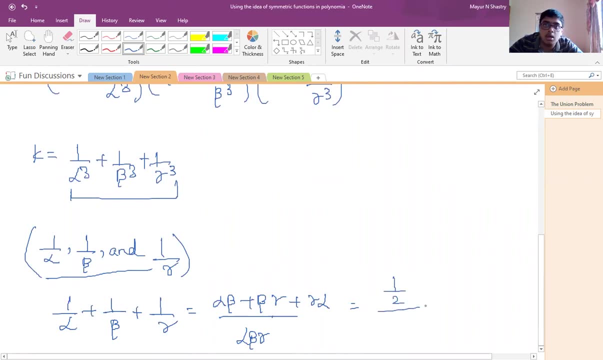 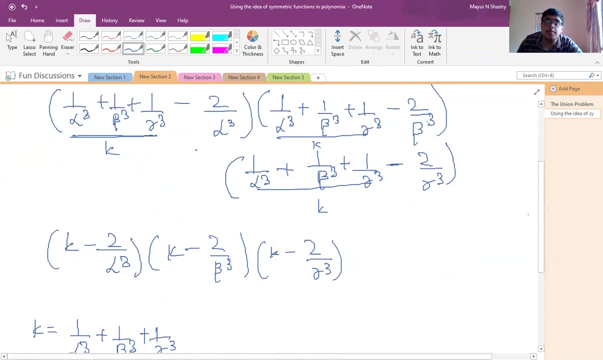 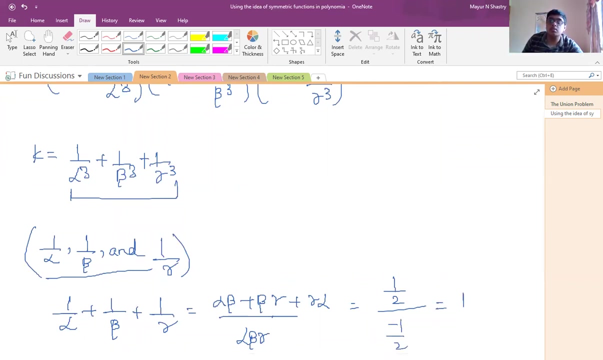 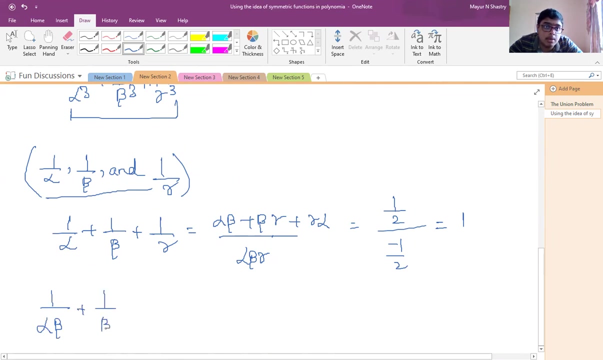 beta gamma plus gamma alpha. it's using vieta's relations. it's uh, one by two right. and what about alpha beta gamma? alpha beta gamma is going to be negative, one by two right. so this is going to give you one. then we need to calculate this: one by alpha beta plus one by beta gamma plus one by gamma alpha. 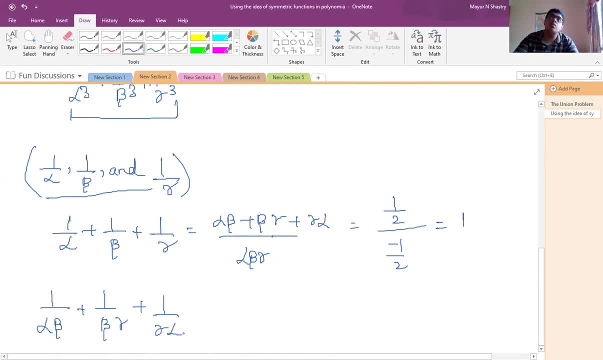 this is the why am i doing this? why am i calculating this? this is how we construct the polynomial with roots: one by alpha, one by beta and one by gamma. it's very much simplified using beta's relations. so that is what we are going to do. so this is going to give you: once you take the lcm, you'll get alpha- beta, alpha plus beta plus gamma. 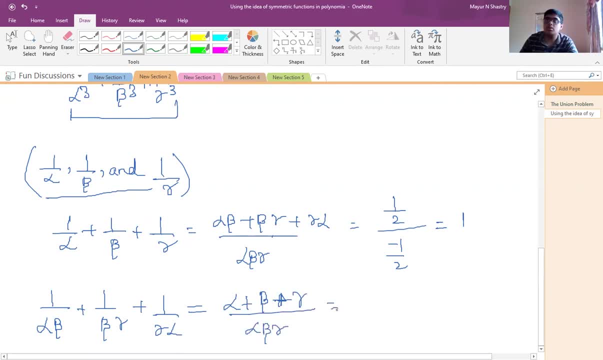 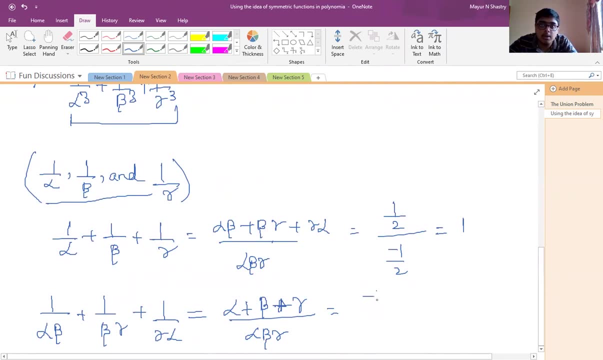 divided by alpha beta gamma, that's going to give you the. c was alpha plus beta plus gamma. that is a negative one by two. and again, even alpha beta gamma is negative one by two. that's going to give you one that is product of the roots. the product of the roots, that is one by alpha beta gamma. 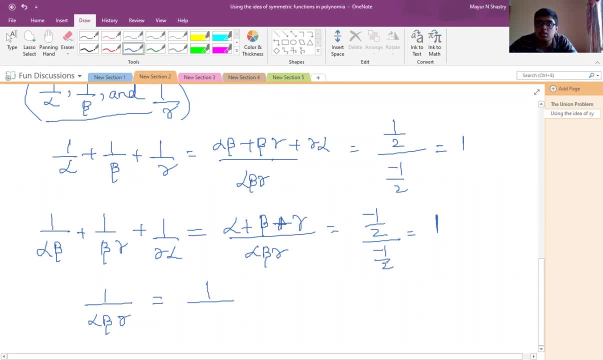 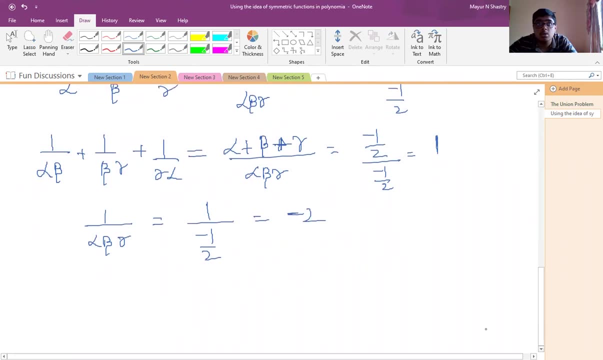 that is going to be. the product is negative one by two. so this, yeah, this becomes minus two now. so this is going to be our x square coefficient. so it's going to be something like this: we're going to have the polynomial to be x- cube, x, cube. 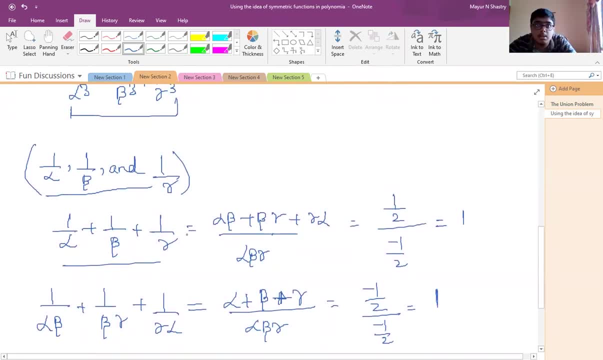 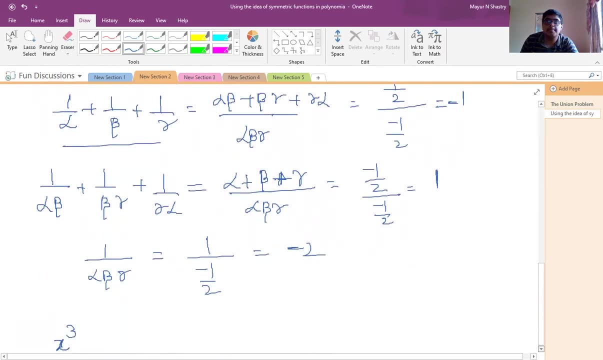 uh, a small mistake. one by alpha plus one by beta plus one by gamma is supposed to be, uh, negative one, this small mistake. so yeah, so now we have this one here. so so now it becomes x cube plus x square, a plus, because when we use vieta's relations it's a minus b by a. 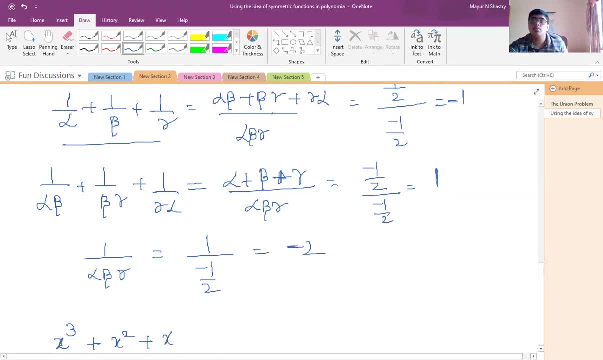 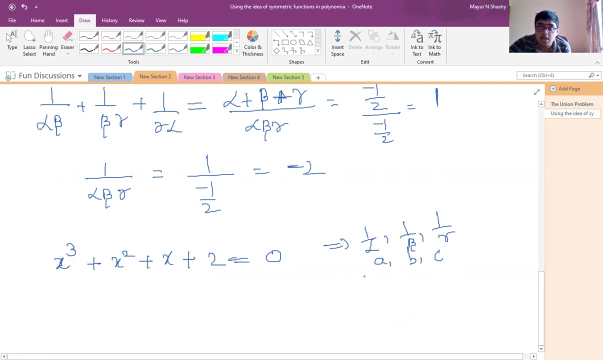 and now this is just a one because it's c by a. now negative, of negative two, that's plus two because it's minus d by a in beta solutions. so this is the polynomial with roots, one by alpha, one by beta and one by gamma. limits a, b and c, because it's harder to always write it as reciprocal. So, since there are the 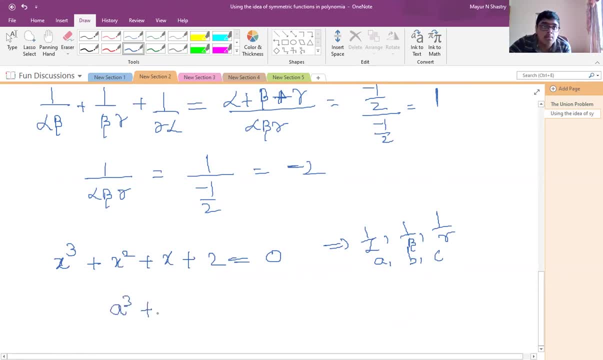 roots of this equation. what can I write? a cube plus a square plus a plus two has to be equal to zero. That's the direct consequence of a being the root of it. Then b is the root of this, so we get b cube plus b square plus b plus two to be equal to zero. and similarly, even c is a root, so we get: 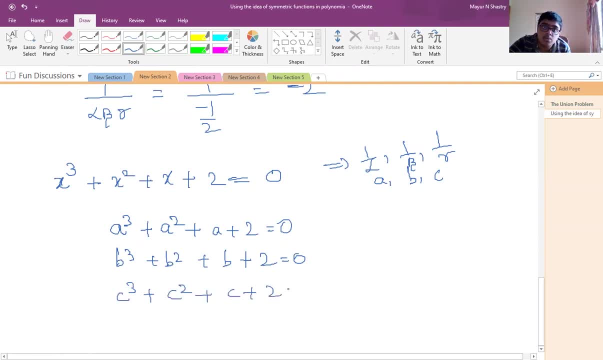 c cube plus c square plus c plus two, to be equal to zero. So actually, what do we want? We want one by alpha cube plus one by beta cube plus one by gamma cube, and you see that it's just a cube plus b cube plus c cube. 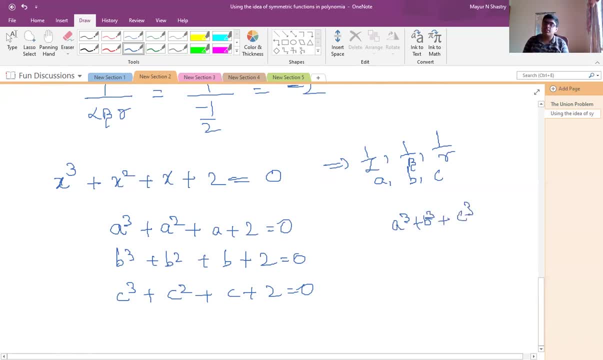 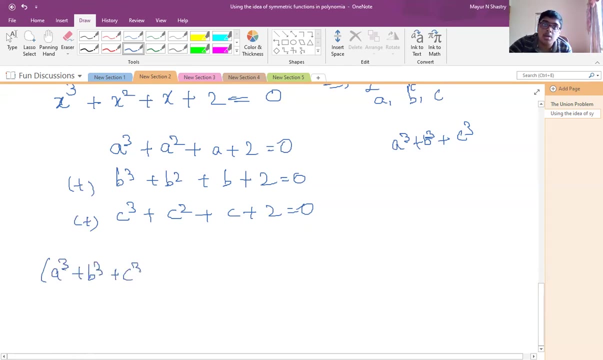 So how do we get that now? How do we get it from these three equations? That's the trick: Add them, add them up, So that's what symmetric function says. So we get a cube plus b, cube plus c, cube plus a. square plus b, square plus c, square plus a plus b plus c plus six, two times three. that. 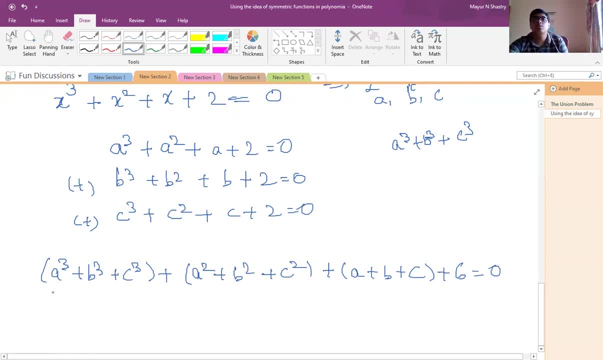 equals zero. So we get a cube plus b cube plus c cube. that is our k and we usually represent this as sigma of a cube. Sigma of a cube would imply that it's a cube plus b cube plus c cube, and we can write this as: 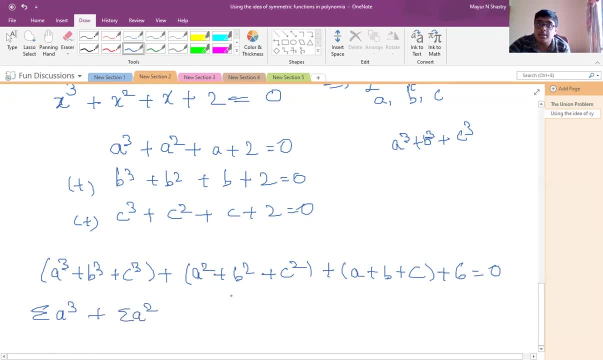 sigma a square, and this is written as sigma a, and this is f plus six equals zero, So this is just the way of representing it, Which will make it more quicker to apply it. You see this? You just write it as sigma a cube plus. 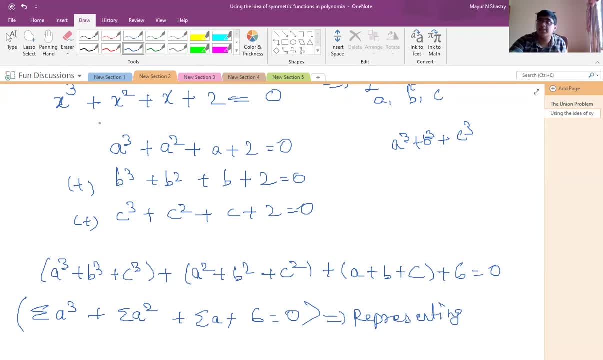 sigma a square plus sigma a plus two times six equals zero. You can directly see it from the equation. It's a direct step. but from where does it come? You write this down like this: The roots of the equation are a, b and c. So we have a cube plus a square. plus a plus two equals zero b cube. 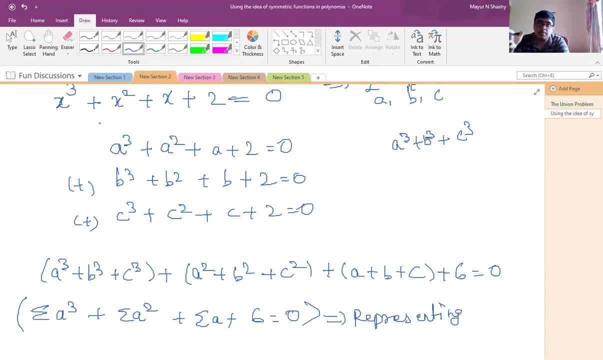 plus b, square plus b plus two equals zero. c cube plus c, square plus c plus two equals zero. and we add them up, So that that's how we get the, how we do the procedure, and once you get enough practice of this, you can write it directly in. 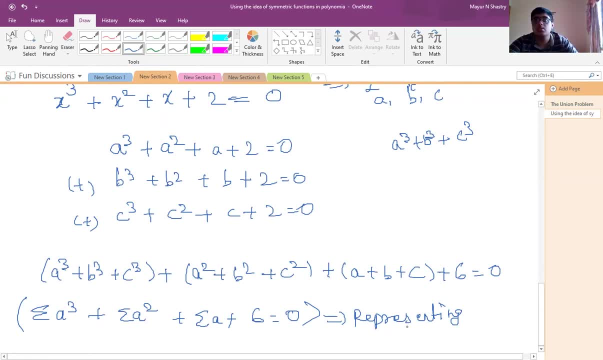 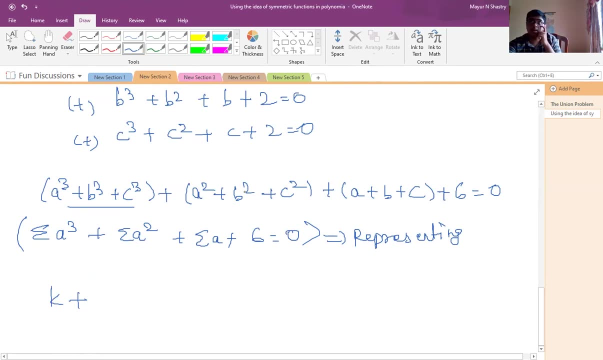 here. So now I'm going to write this as just k, because that's what we want to find, and this can be written as We don't want: a square plus b, square plus c square, but we know an identity. What's that identity? So I'm going to use this identity: a plus b plus c, the. 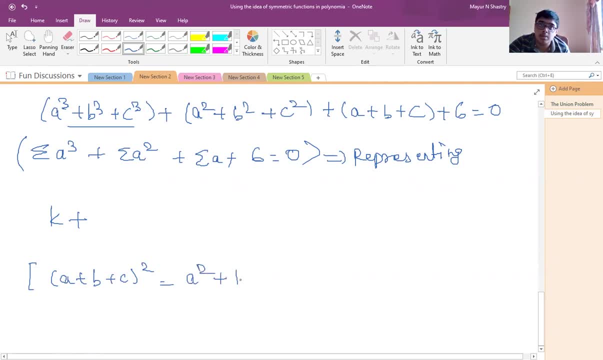 whole square is equal to a square plus b square plus c square, plus two times of a, b plus b, c plus c a. This, of course, is a very nice relation which we are going to use. So, again, we're going to use this so I can write a square plus b square plus c square to be a plus b plus c the whole square. 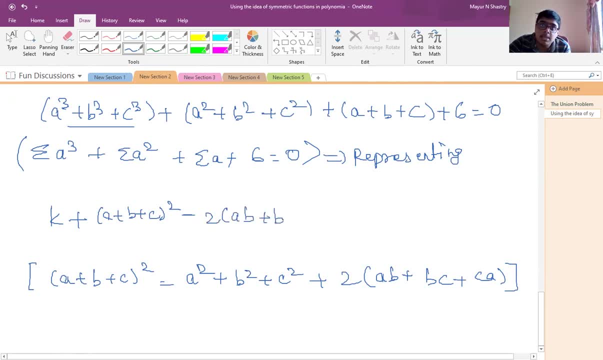 minus two times a, b plus b, c. So it is a plus b plus c plus c, a plus a plus b plus c plus six equals zero. and now they're almost it. And what is a plus b plus c? the whole square? That's one by alpha plus one by beta plus one by gamma, the whole square Class. we already. 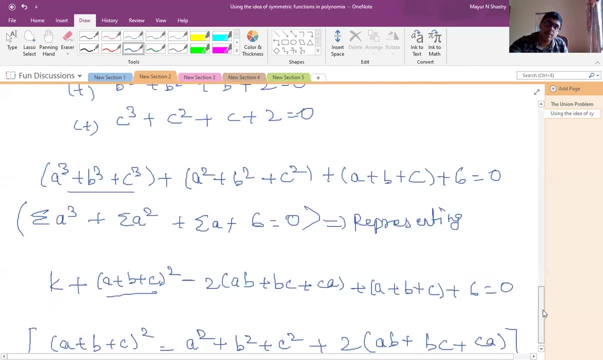 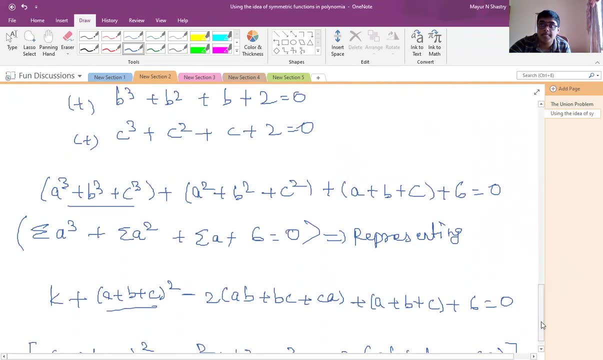 calculated what's one by alpha, That's one by beta plus one by gamma, plus one by negative one. So we have k plus negative one, the whole square, because it is zero. So at this point we just got one c in and now one b for each. it's given us. 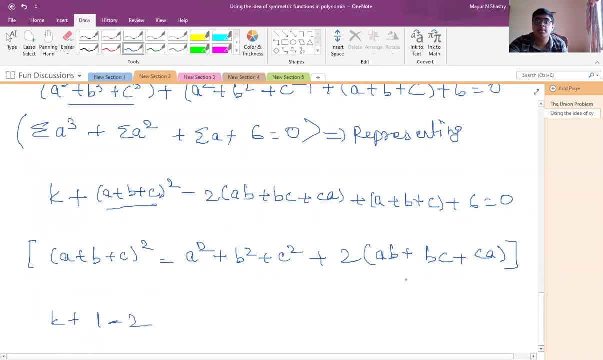 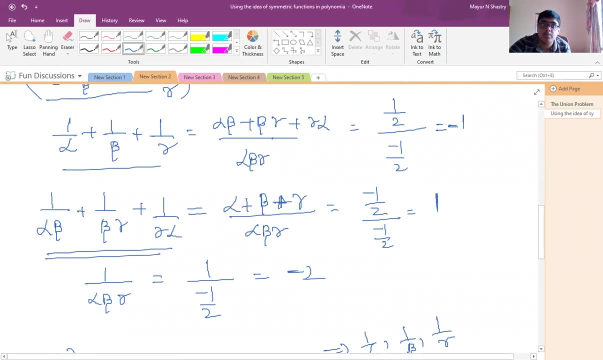 There is another c there Also. we didn't know that there was another c in the previous exercise. square is 1 minus 2 times of a b plus b, c plus c a. that was a b plus b, c plus c a. is this expression? 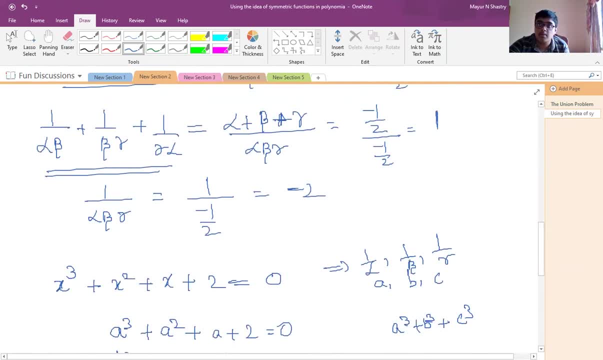 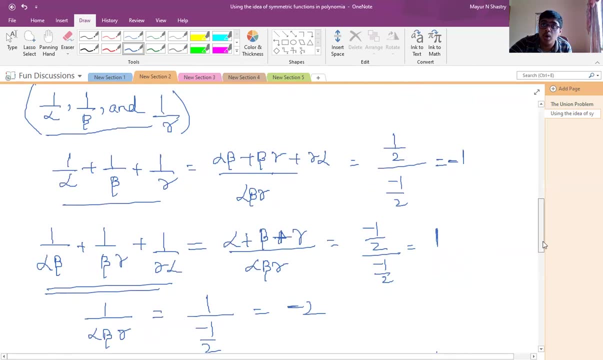 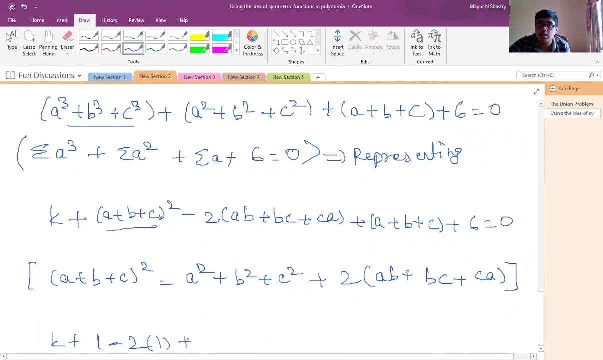 if you realize, since a is 1 by alpha, b is 1 by beta and c is 1 by gamma, you could just substitute and check. so this is going to give us 1. so minus 2 times 1, plus a, plus b plus c, that is negative 1. 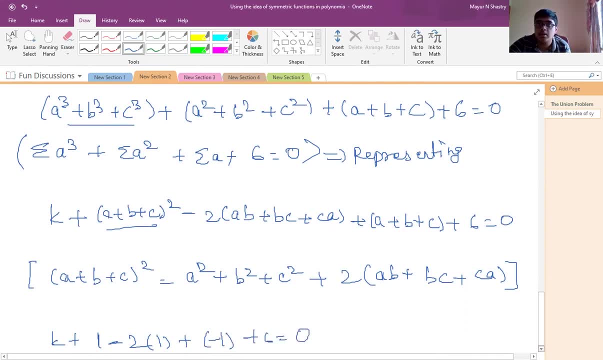 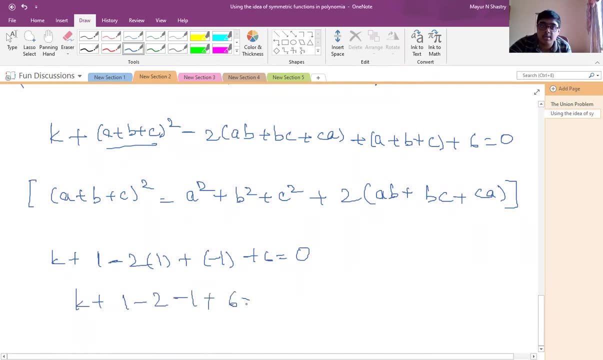 plus 6 equals 0, right? so then we have k plus 1 minus 2 minus 1 plus 6 equals 0 and we have a 1 minus 1 getting cancelled. we have k plus 4 equals 0 and we have k equals minus 4 important. 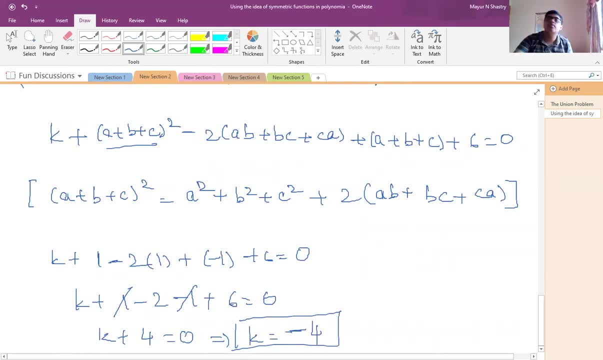 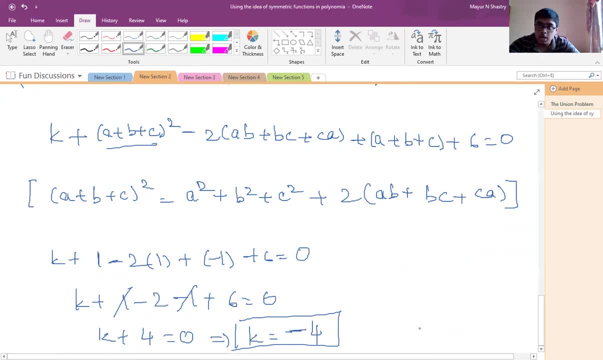 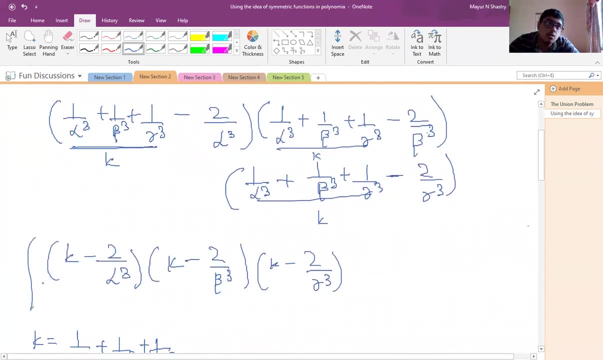 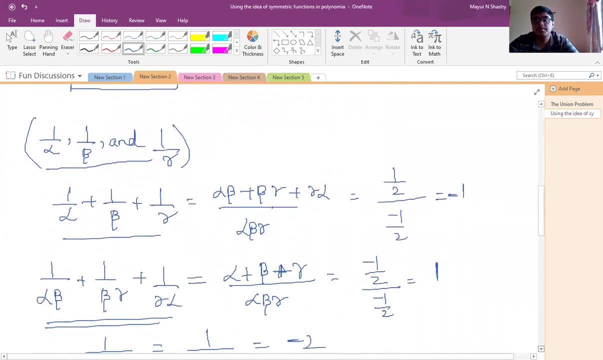 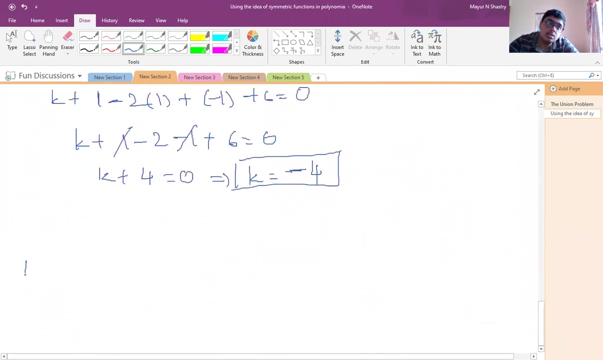 cube is actually negative 4, so now a big leap. what was our expression this right? we found this out and we know that k is minus 4 now, so let's put k is minus 4 in that expression. yeah, so the expression, the expression was k minus 2 by alpha cube times k minus 2 by beta cube times k minus 2 by gamma cube. 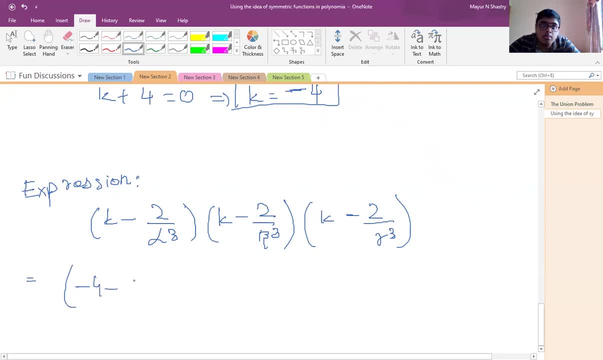 so and k is minus 4, so minus 4 minus 2 by alpha cube times, minus 4 minus 2 by beta cube times, minus 4 minus 2 by gamma cube. so now we can pull minus 2 out from each of the product terms. so we are going to be left with 2 plus 1 by alpha cube times 2 plus 1 by beta cube. 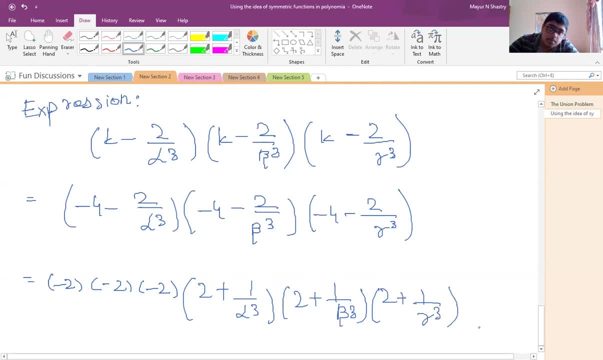 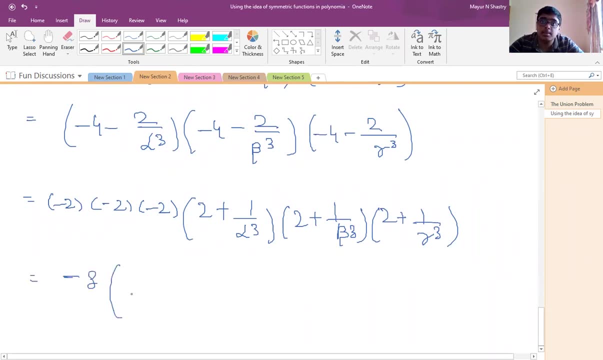 times 2 plus 1 by gamma cube, right, so this is going to give us minus 8 times. it's not very hard to expand this. we won't get uh. you know we would get uh 8 terms, that's all. so when we expand these two first, we get 4 plus 2 by beta cube, plus 2 by alpha cube plus 1 by 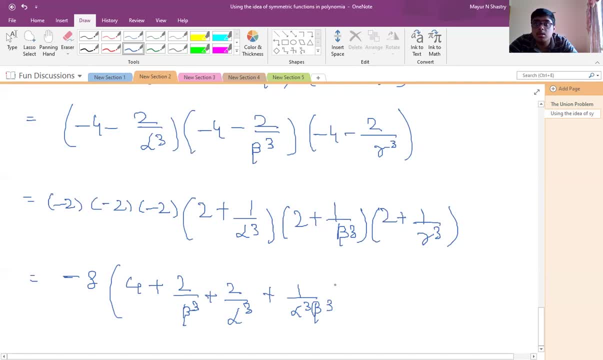 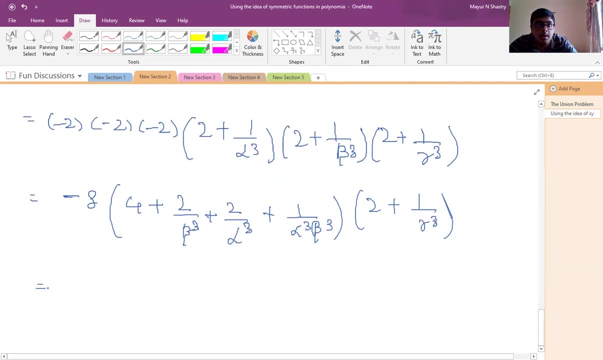 alpha cube, beta cube, then this multiplied by two plus one by gamma cube, so then we have a minus eight times so four times two. that is eight plus four by gamma cube and two by beta cube times two. so that's plus four by beta cube and we get plus two by beta. 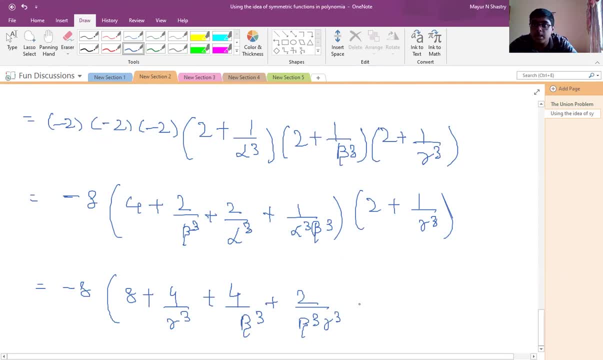 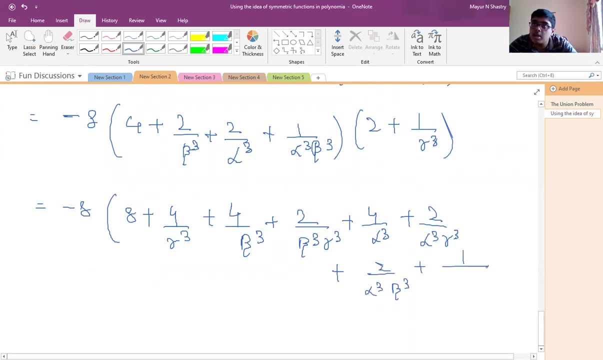 cube, gamma cube. then we get a plus four by alpha cube, then we have plus two by alpha cube, gamma cube, and a plus two by alpha cube, beta cube, and then finally a plus one by alpha cube, beta cube, gamma cube. wonderful, we've got this. so now what do we have? minus eight times eight, plus, 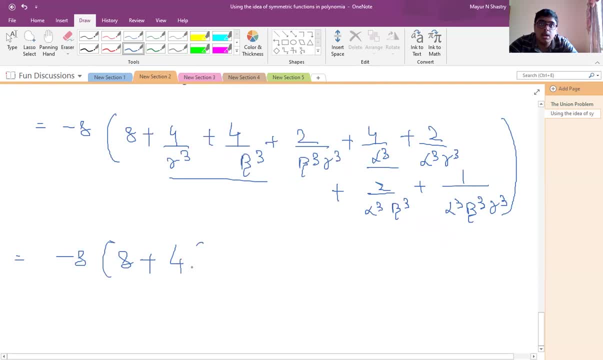 let's group these terms. so four common. and what do we have? one by alpha cube plus one by beta cube, plus one by gamma cube, and we know what this is. that's negative four, the value of k which we calculate. then we have plus two times one by alpha cube, beta cube, plus one by beta cube, gamma cube. 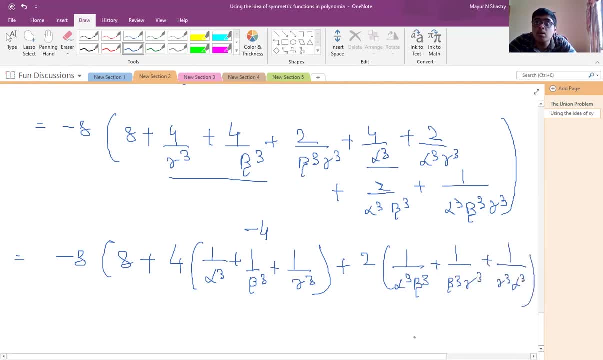 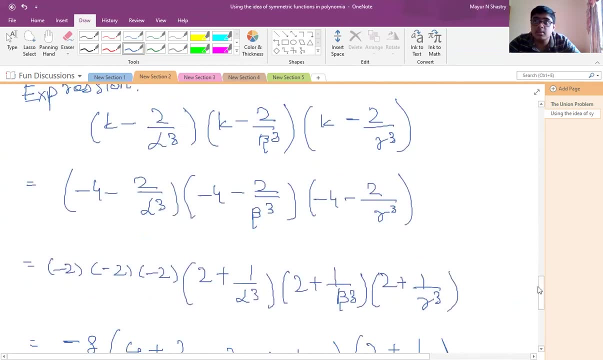 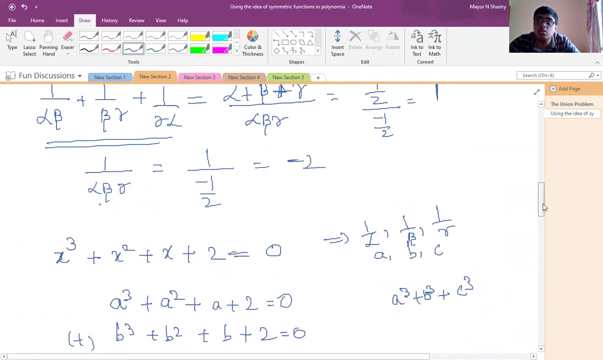 plus one by gamma cube, alpha cube plus what is 1 by alpha cube, beta cube, gamma cube. so realize that 1 by alpha beta gamma. what did we find out? that the value of 1 by alpha beta gamma is negative two. so what would be 1 by? 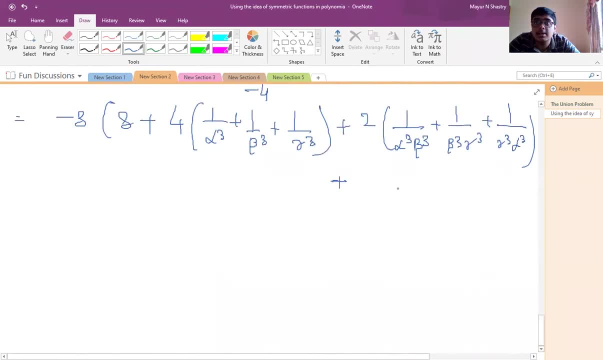 alpha cube, beta give gamma cube, that would be negative eight. wow, that's nice. and what's more nice is that this minus eight and this 8 is cancel. so now what we have? so we have minus minus 8 times, 4 times minus 4, that is minus 16 plus 2 times, so we can take the LCM here. 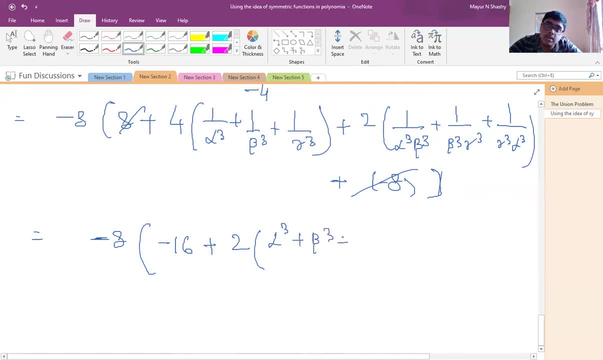 you notice that you get alpha cube plus beta cube plus gamma cube. divided by alpha cube, beta cube, gamma cube, and again 1 by alpha beta gamma was negative 2, so 1 by alpha cube, beta cube, gamma cube would be negative 8, so we can write it as minus 8 times minus 16 plus. 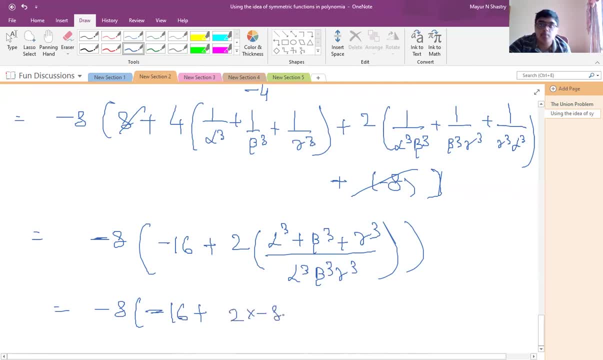 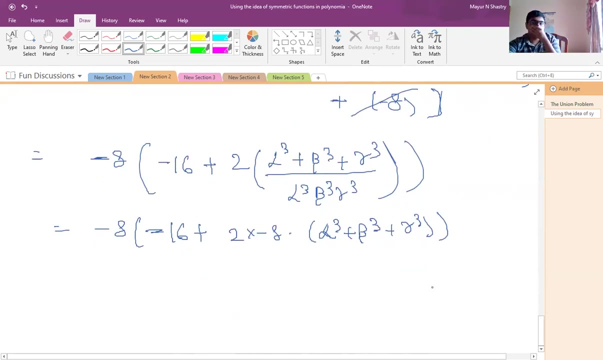 so 2 times minus 8, it would be times alpha cube plus beta cube plus gamma cube. so yeah, so what do we have to find? so what do we have to find? is that this expression? what is this expression? we haven't calculated it yet. so our next goal: 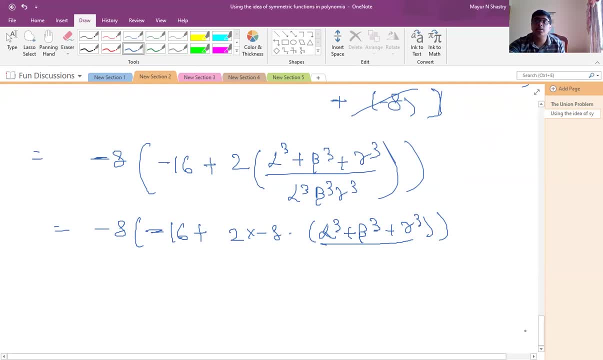 would be to calculate that, that what is alpha cube plus beta cube plus gamma cube? let's see what that is and again realize that alpha cube plus beta cube plus gamma cube is in fact a symmetric function, because if you replace any two of alpha, beta or beta, 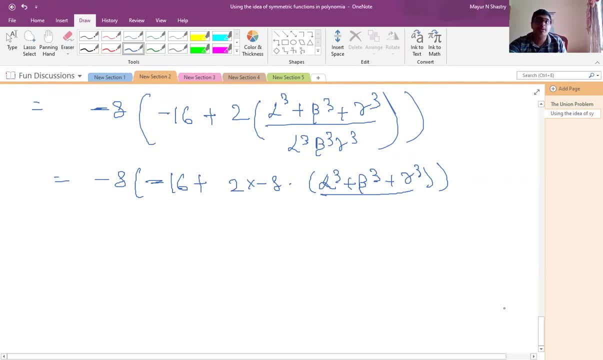 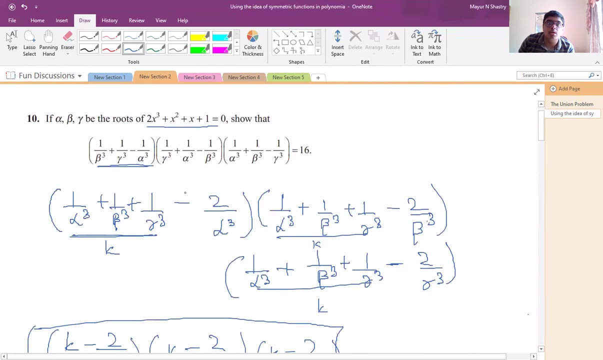 gamma or gamma alpha, you would get the same expression. it doesn't change. so now, alpha, beta and gamma are the roots of this equation. the given equation, what was given in the problem: 2x cube plus x, squared plus x plus 1 equal to 0. 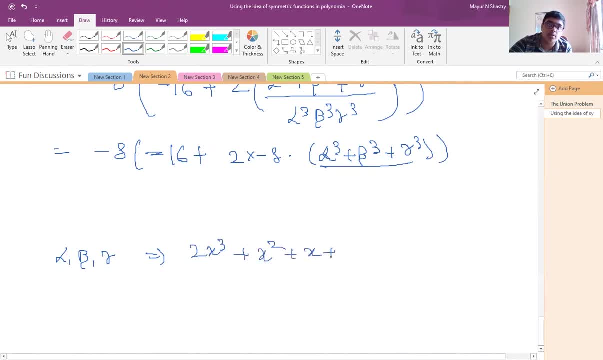 2x cube plus x squared, plus x plus 1 equals 0.. so now let us see what we can do. so, since alpha is a root, we have 2 alpha cube plus 2 alpha. sorry, not a 2 alpha squared, it's just 1 alpha squared. 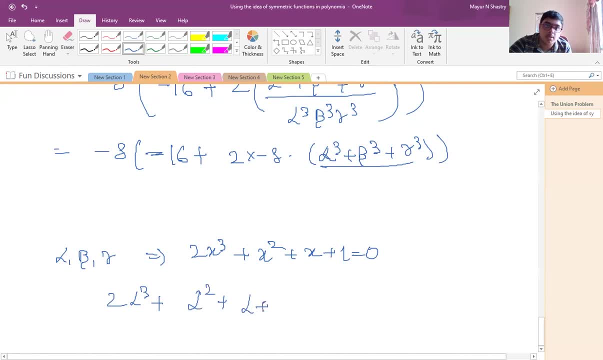 1 alpha squared. so alpha squared plus alpha plus 1 equals 0. we have 2 beta cube plus beta squared. plus beta plus 1 equals 0, and again you could do this directly if you have practice, 2 gamma cube plus gamma squared plus gamma. 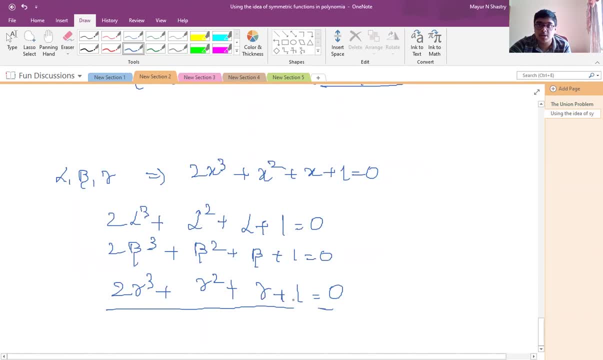 plus 1 equals 0.. I'm doing this so that you realize how symmetric functions to work actually. so again we had all these equations. as usual, you get twice of alpha cube plus beta, cube plus gamma, cube plus alpha square plus beta, square plus gamma, square plus alpha plus beta plus gamma. 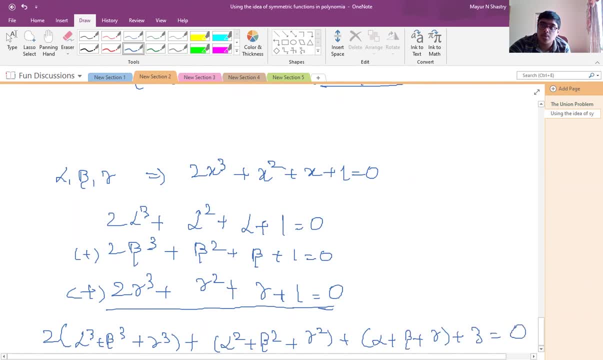 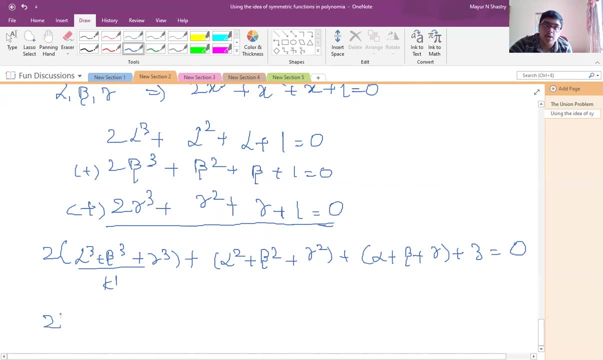 and plus 3, this equals 0, and then let us call this as sum k prime 2k. prime plus alpha square plus beta square plus gamma square can be written as alpha plus beta plus gamma, the whole square minus twice of alpha, beta plus beta gamma plus gamma alpha, and this is just alpha plus beta plus gamma plus 3, and 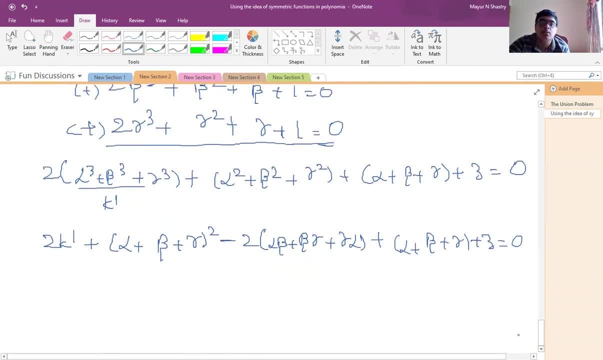 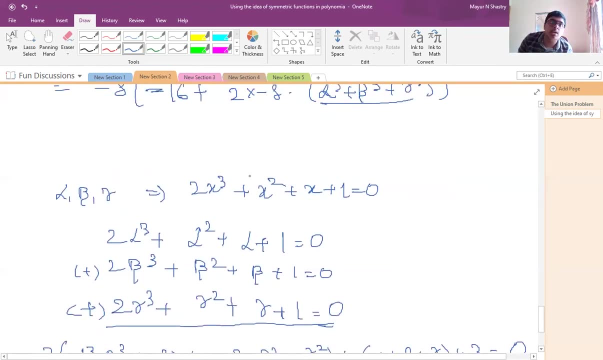 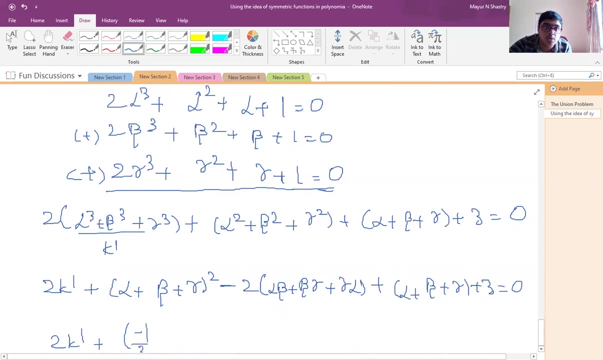 three and this equals zero. And what is alpha plus beta plus gamma? From again, using Weierthaus relations, it's negative one by two. So we get a negative one by two, the whole square minus twice of alpha beta. 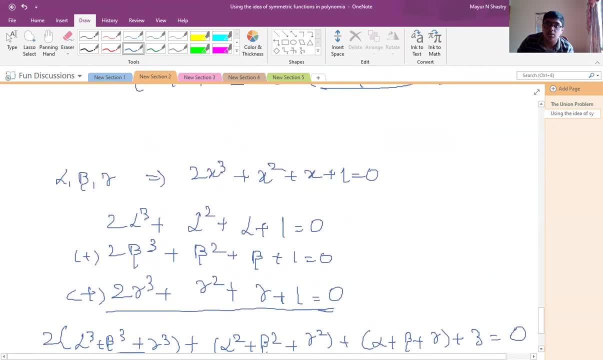 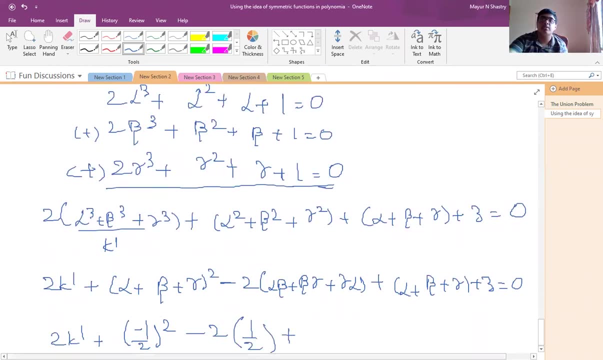 plus beta, gamma plus gamma, alpha. What's that? That's going to be one by two. again, from Weierthaus relations, We're going to get one by two plus alpha plus beta plus gamma. This now we saw that it's negative. one by two. 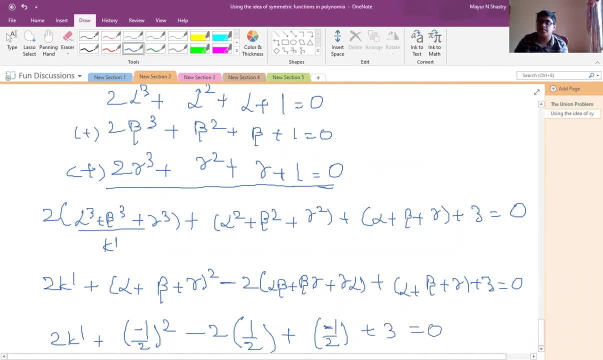 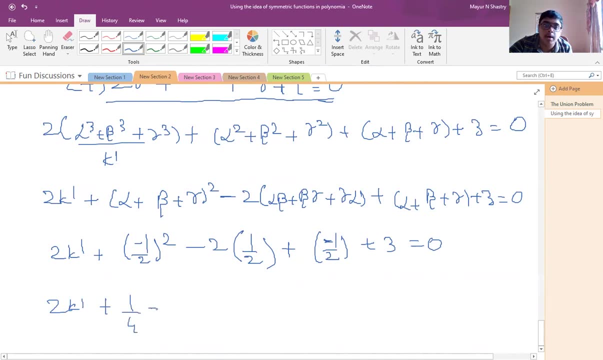 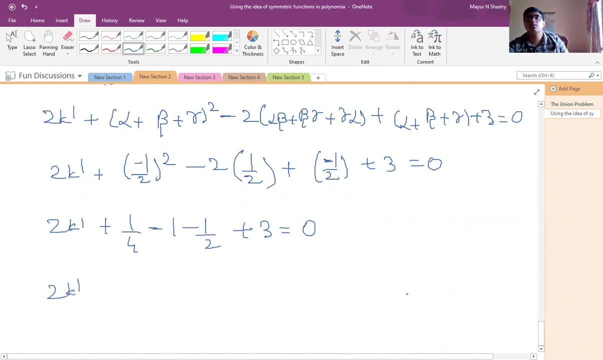 and then plus three. This should equals zero. So then we have two k dash plus one by four minus one and minus one by two plus three equals zero. So we get two k dash minus the half. what do we have? So this is one by four minus half, would give you. 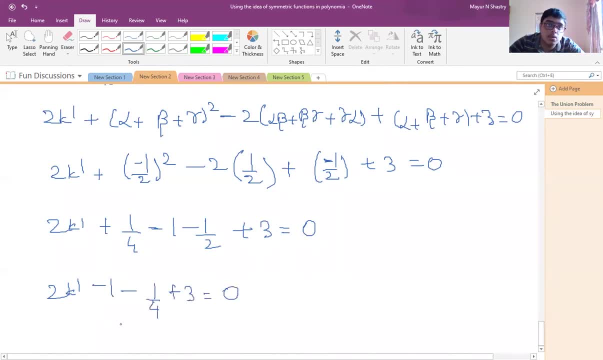 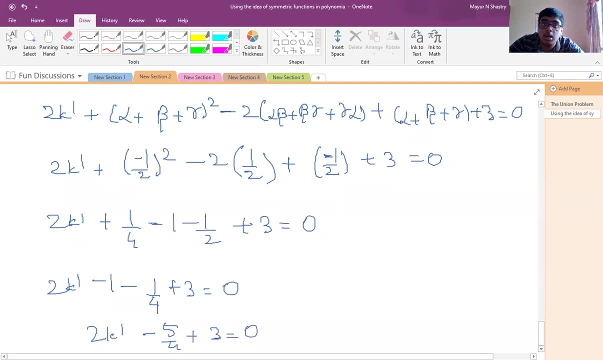 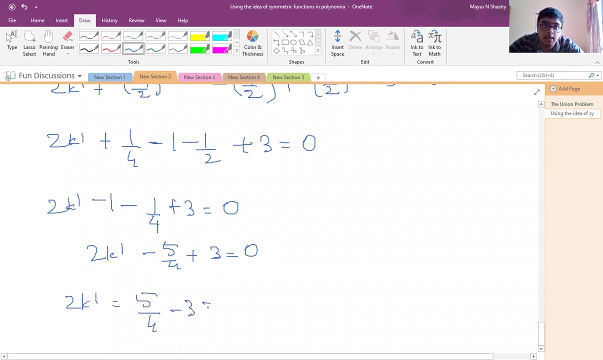 minus one by four, then plus three equals zero. So we get two k dash minus five by four. plus three equals zero, and we get that two k dash is in fact five by four minus three. That is going to be five minus 26.. 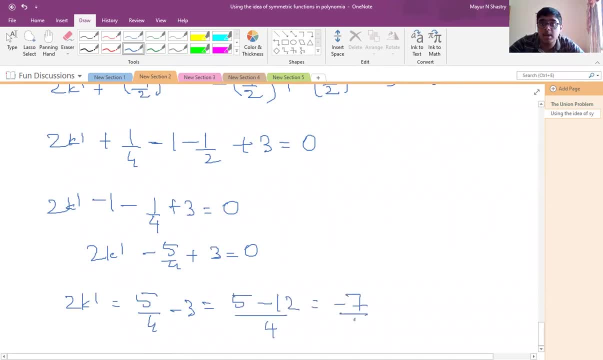 divided by 4. so that's going to be minus 7 by 4. so what's going to be k dash? it's going to be minus 7 by 8. okay, so sort of a bit difficult kind of a value to you know, accept because you. 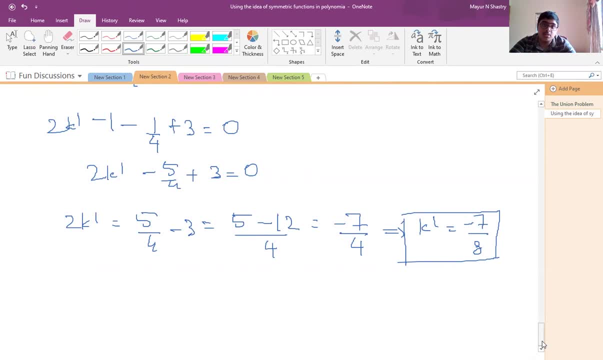 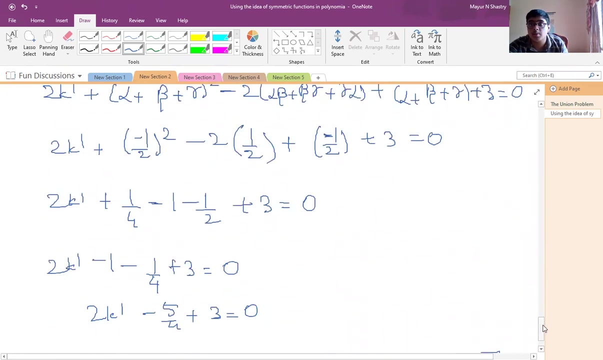 may tend to see that, oh, it might not give us the answer as 16 because there's a fraction, but you would see that it gets cancelled once we do it. so k dash is negative 7 by 8. and what? what? what was the expression? simplified to this expression? minus 8 times minus 16. 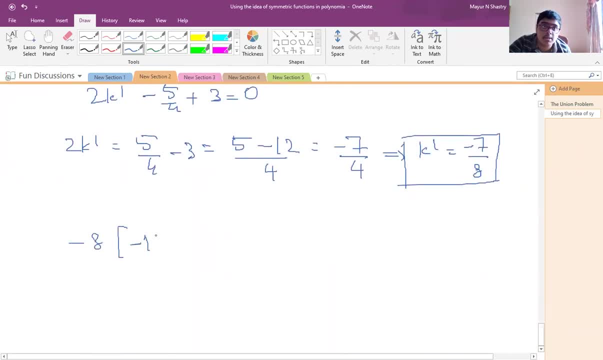 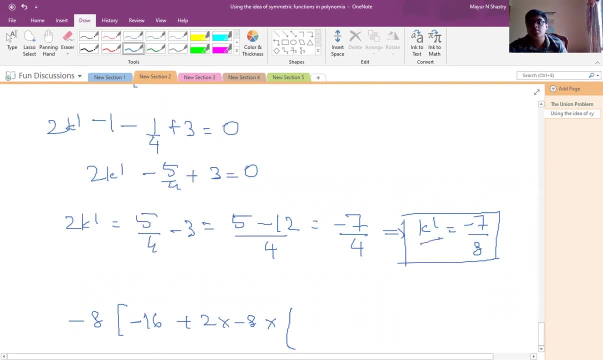 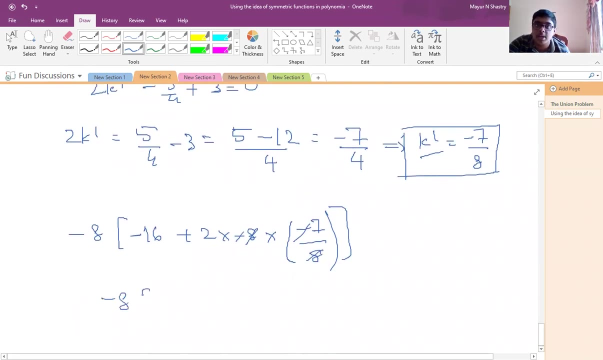 it is going to be this: that is what we assumed as k prime. that's going to be negative: 7 by 8. so what do we have? this minus and a minus becomes plus, then 8 and 8 gets cancelled. so what do we have? minus 8 times minus 16, plus 2 times 7, that is plus.